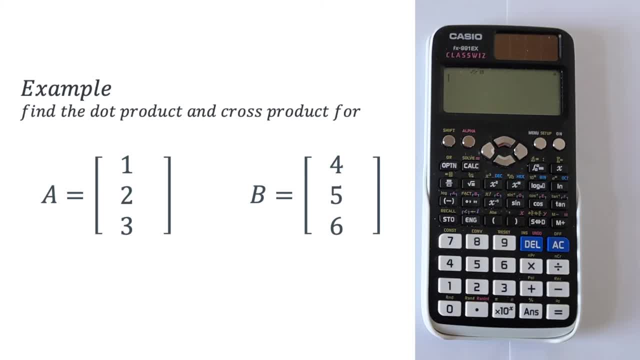 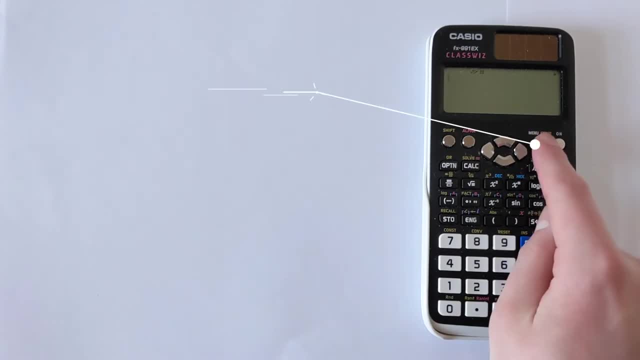 B is going to be 4, 5 and 6.. And to find the dot and cross product you have to first put your calculator into the correct mode. So we're going to look at vector mode. So we're going to press the button here for menu and then if you go down you can see you've got option 5, which is 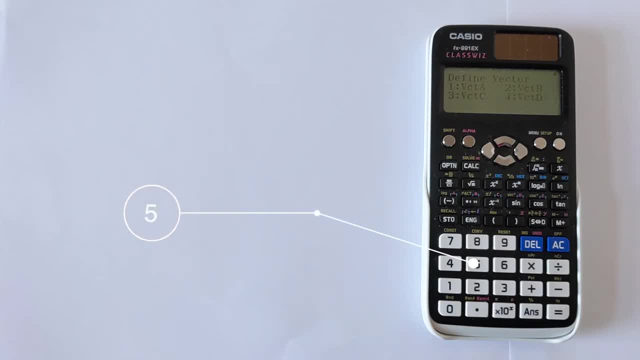 vector. So we press 5 and we're now into the correct mode And this will let you define the vector, which is our next step. So we're going to define vector A and then define vector B to input these values into the calculator. So let's select option 1 for vector A, Then it'll ask for the. 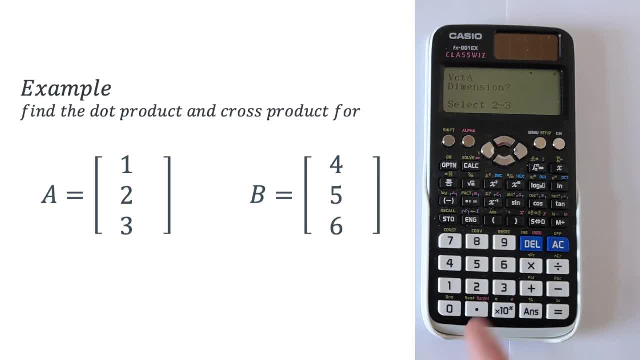 dimension. We've got three numbers in each of the vectors, so we're going to select option 3.. So that's 3 for the dimension. Then we are going to input the vector. So we've got 1 equals, 2 equals, then 3 equals. 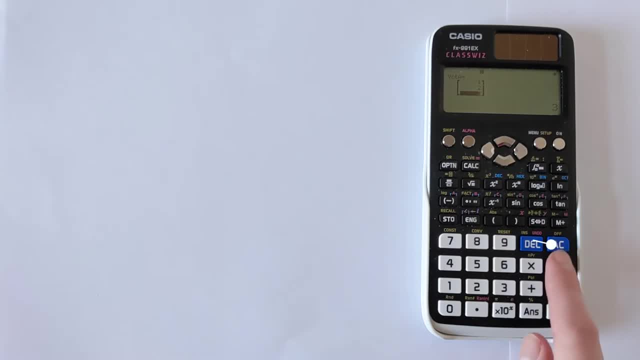 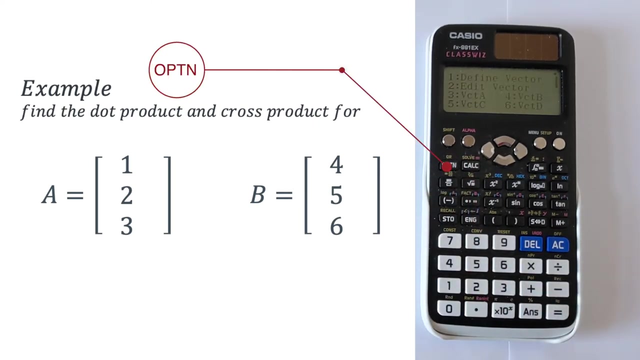 Once you've put in your first vector you have to press AC and then that brings you to this screen and you can see that vector is shown telling you you're in the right mode To enter vector B. you have to follow a slightly different process. So you select the option button here, Then you have 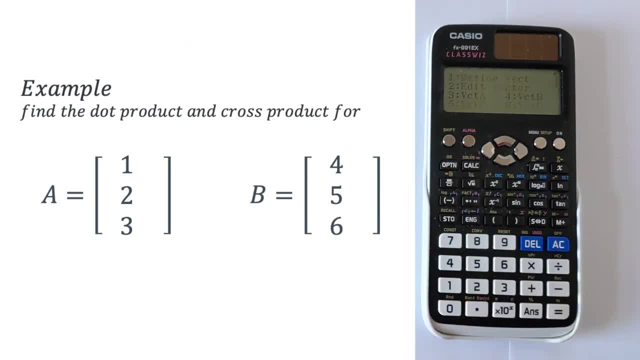 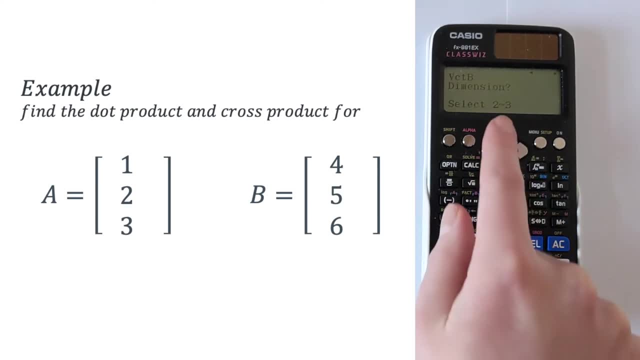 to go back into define vector on option 1.. Then that gives you the chance to define the vector B, which is on option 2.. Then we can select the dimension. Again, this is going to be 3 because we've got three numbers. Then we can go: 4 equals, 5 equals, 6 equals And, as before, we press the AC. 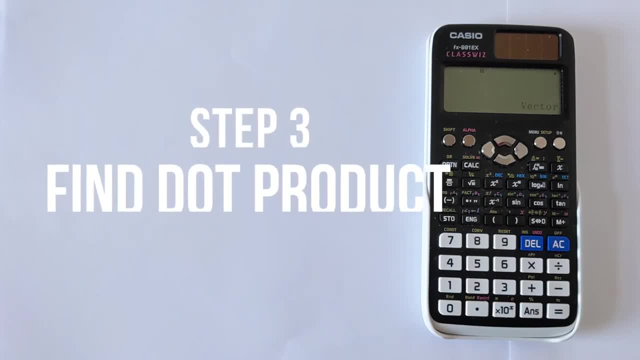 button and then we come back to this screen. Now we can do the calculation. So let's start by doing the dot product. So we need to recall vector A and vector B from the memory and access the dot product function, And to do that you press option. 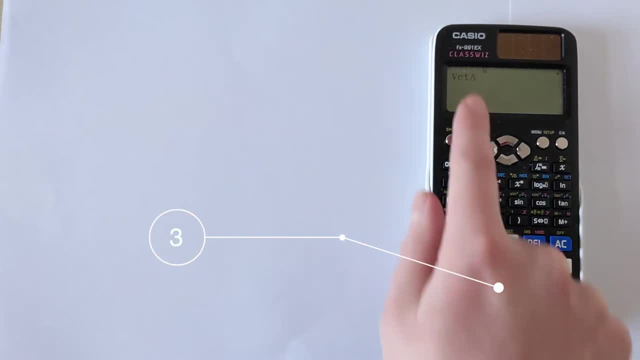 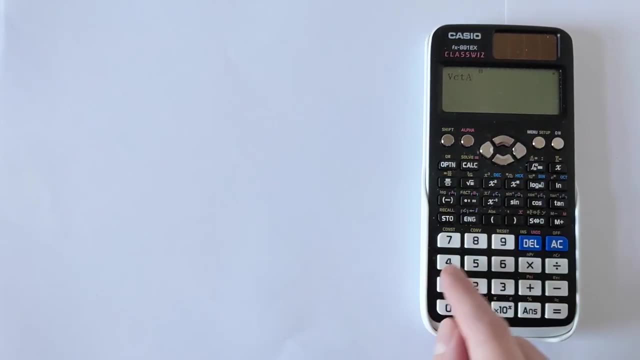 3 will bring up vector A and it shows you VCT A. We want to see VCT for vector A, dot VCT B for vector B, And so we need the dot. So you go option. Then when you press down, you can see.